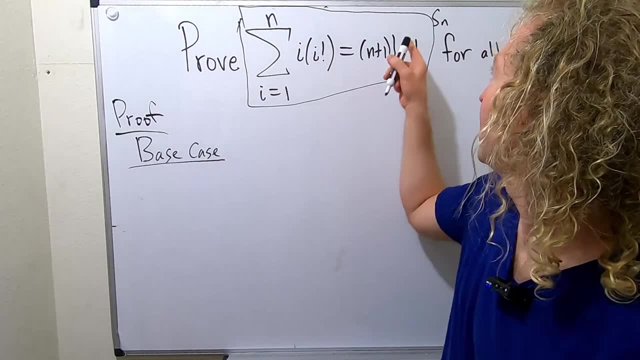 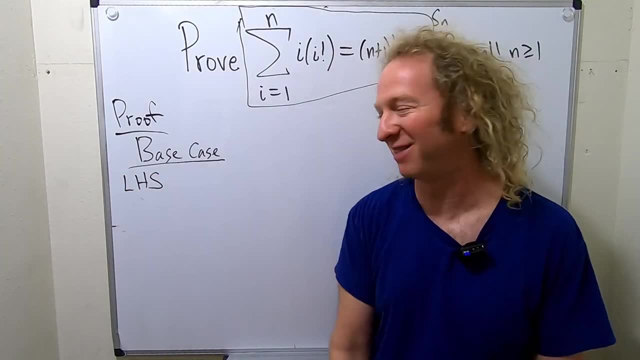 this case that would be 1,, right, So to show that s sub n is true and n is equal to 1.. So let's work out this first. So the left-hand side- I love using this notation: LHS, right, So you replace the n with 1.. This is. 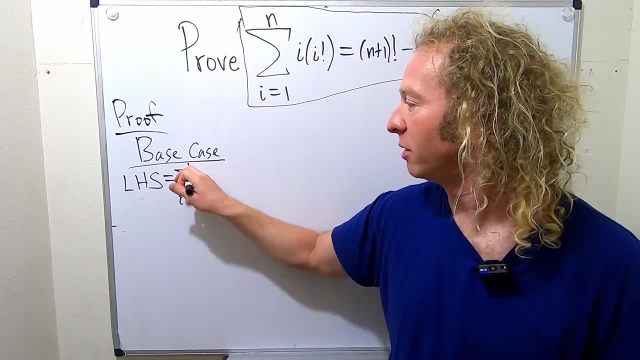 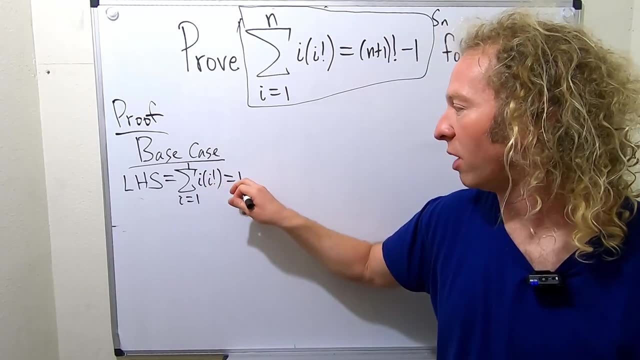 equal to the finite sum, as i runs from 1 to 1, right, Being totally pedantic, i, i factorial, And basically it means you plug in 1.. So you get 1, 1 factorial. 1 factorial is 1.. So you just. 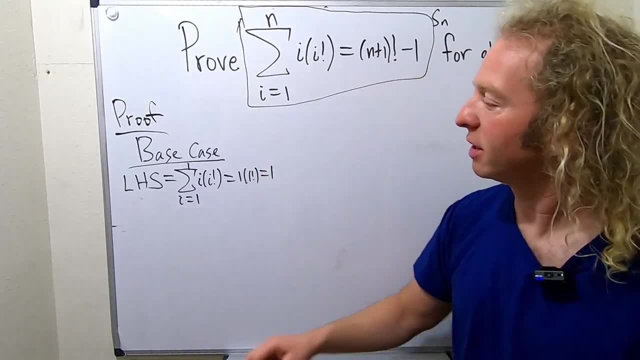 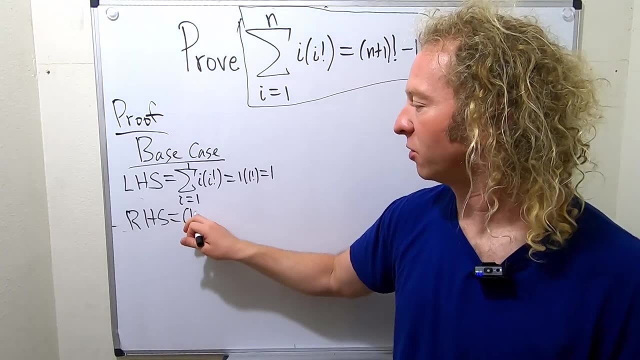 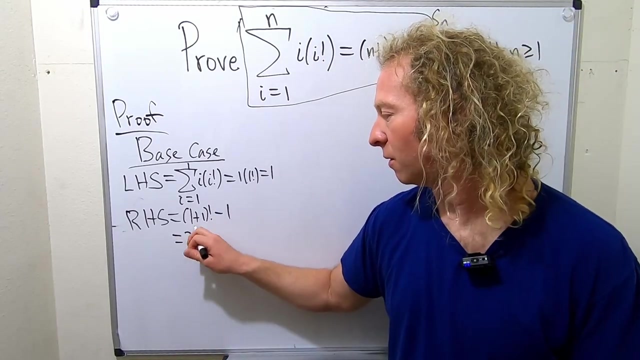 get 1 times 1.. So you just get 1.. Piece of cake. The right-hand side- right-hand side is 1 plus 1, right. So it'd be 1 plus 1 factorial right Minus 1.. So minus 1.. So that's 2 factorial Minus. 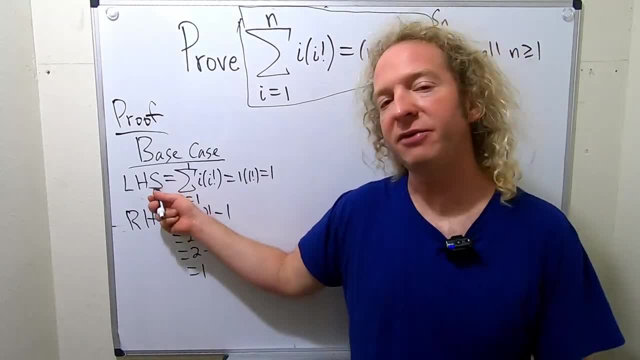 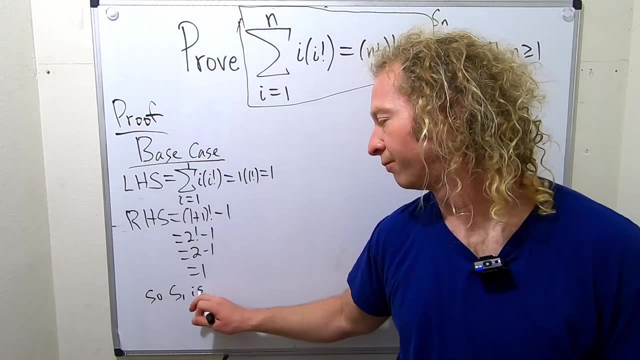 1. So that's 2 minus 1. So that's 1.. So the left-hand side is equal to the right-hand side. So the statement is true and n is equal to 1.. So s sub 1 is true. Good stuff That takes care of. 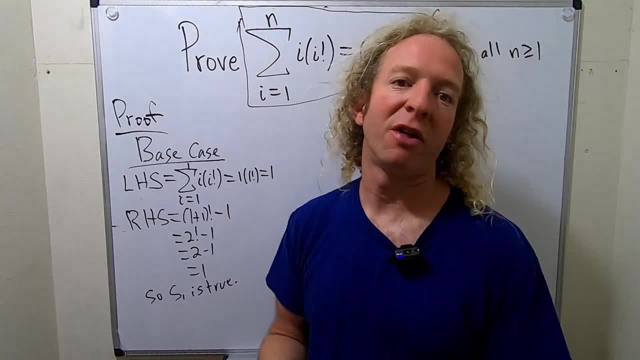 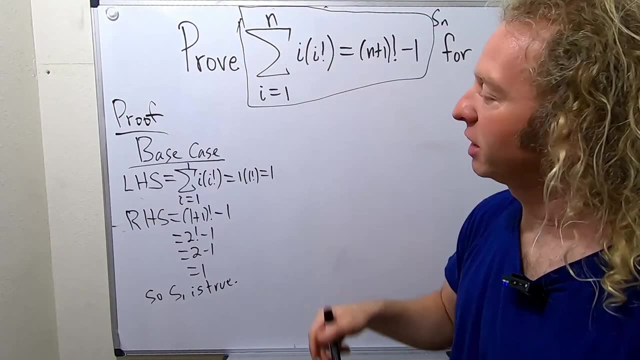 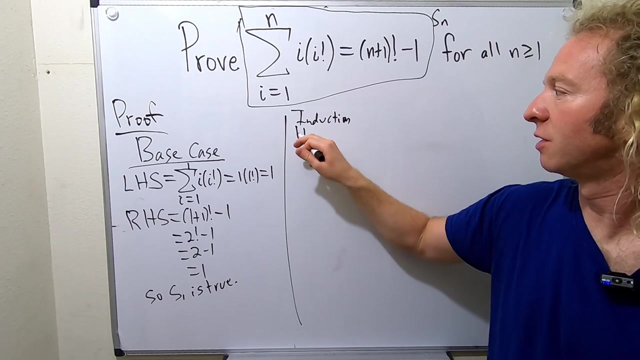 the base case. Piece of cake. Now we get to write down the induction hypothesis. Basically, all we do is we suppose our statement is true when n is equal to k, So we just basically write this down and plug in a k and say it's true. So the induction hypothesis right. We get to say that this is true when n is. 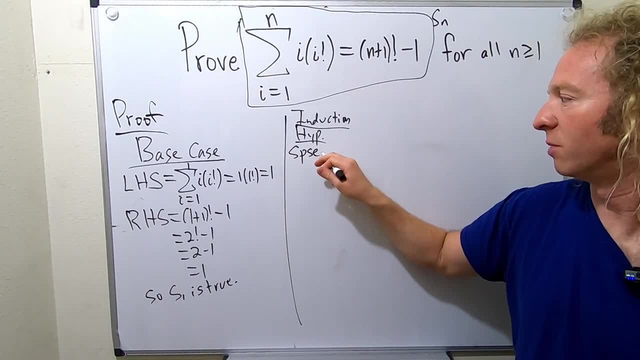 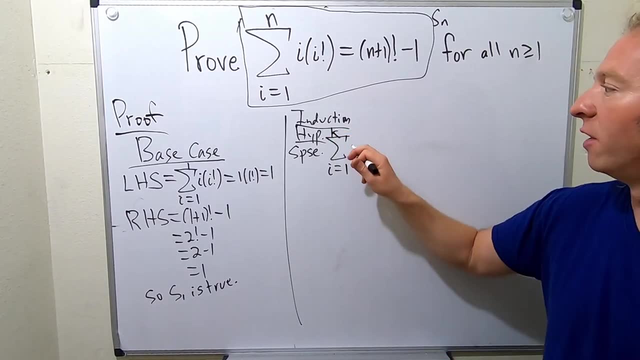 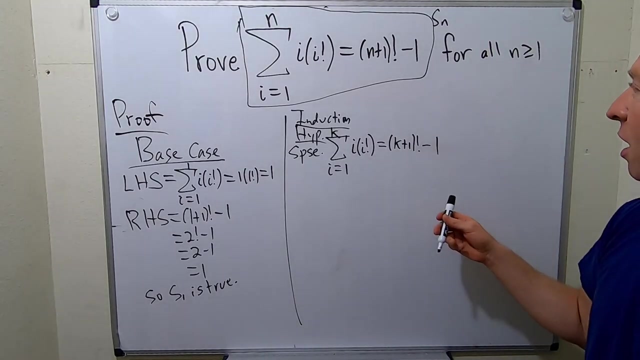 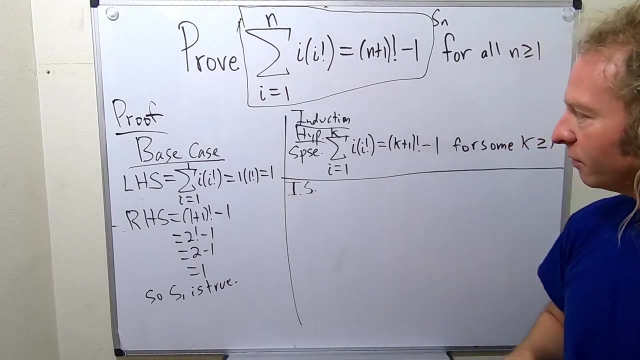 equal to some k. So suppose, suppose that we have this finite sum, as i runs from 1 to k. okay, of i times i, factorial Equal to k plus 1, factorial minus 1.. So we get to assume this is true, All right. so now we have to show that it's true when n is equal to k plus 1.. Oh, and this is for some k. So for some k greater than or equal to 1, right, You're supposed to write that. right, You're supposed to write that. All right, let's do our induction step now. So our induction step is going to put is to save room, Is it to show that this is true when n is equal to k plus 1.. So claim: 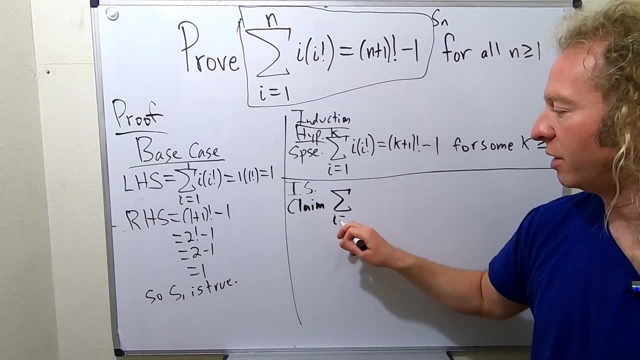 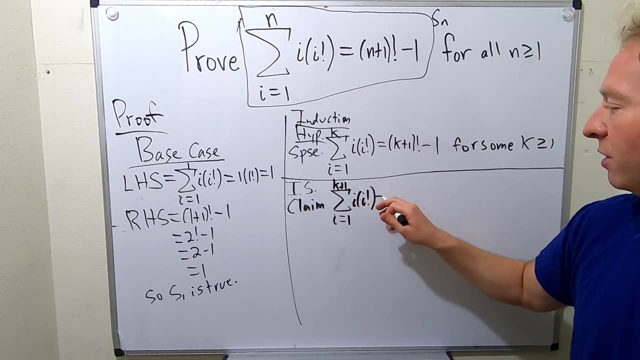 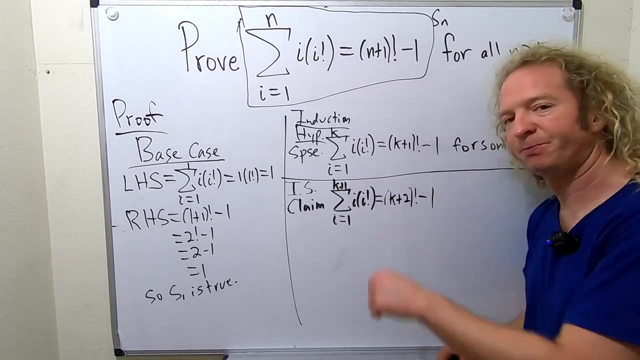 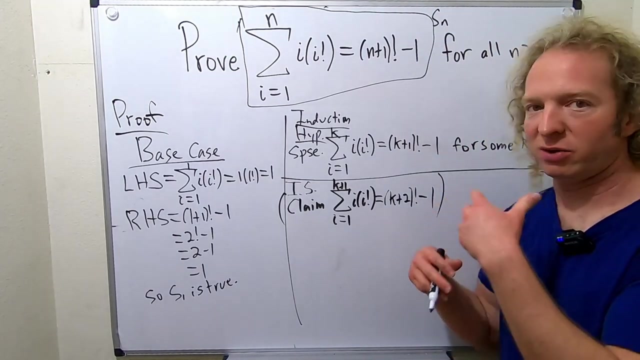 this statement. so the sum from i equals 1 to k plus 1.. I hope this works out. This is i. i factorial equals k plus 1, plus 1 is k plus 2, so we have to show this is a k plus 2 here, minus 1.. So to show this is true. All right, this is the claim. It's not part of the proof, It's what we have to show. It's a really good idea to write down what you're trying to show, because that way you can do the problem Right. You can't do it unless you know what you're trying to do. Okay, so 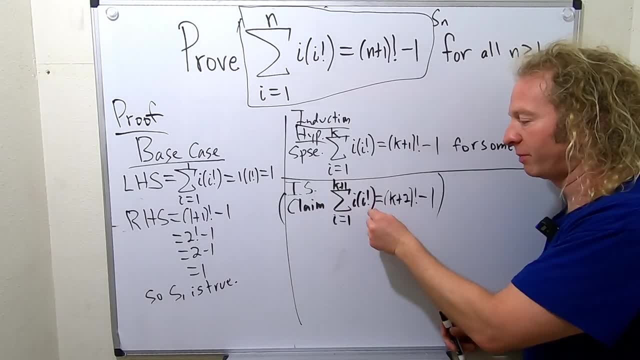 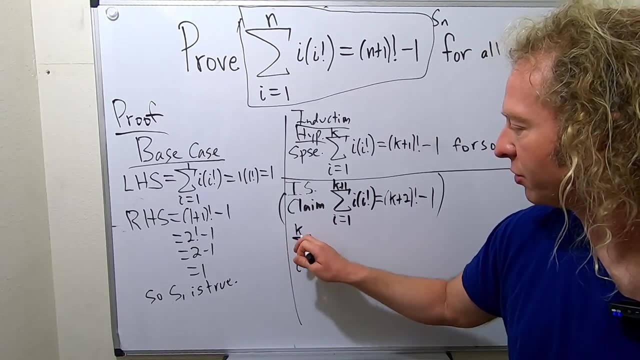 So let's just try to do it the most obvious way possible. We'll start with this and we'll somehow show it's equal to this. So I'm going to start by writing this down: The finite sum as i runs from 1 to k plus 1 of i, i, factorial. 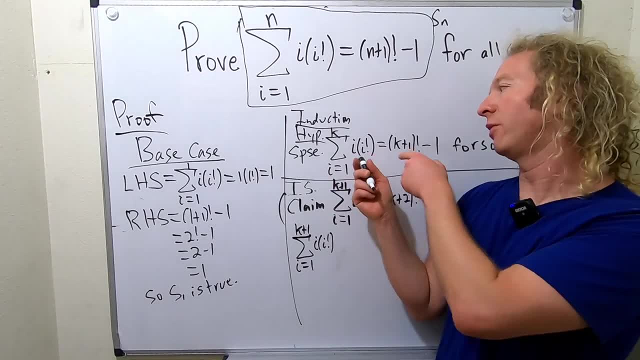 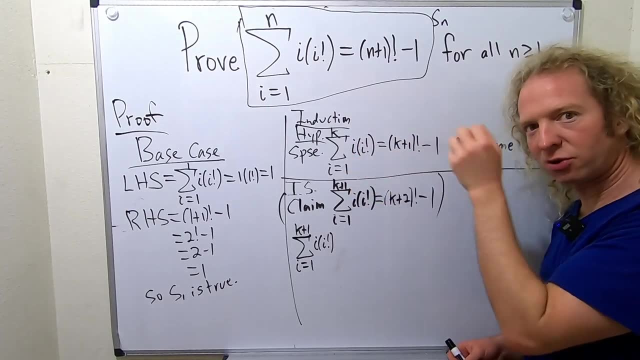 And the natural thing to do is to try to somehow involve this. So in any induction proof you always have to involve your induction hypothesis. You should always use it. That's like the key step in the entire proof. If you manage to use it and you get to the right result, you probably did it right. 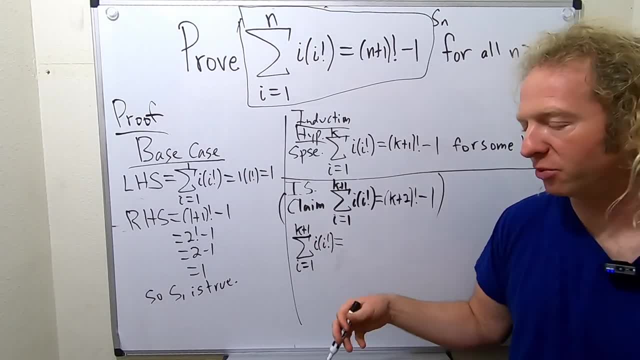 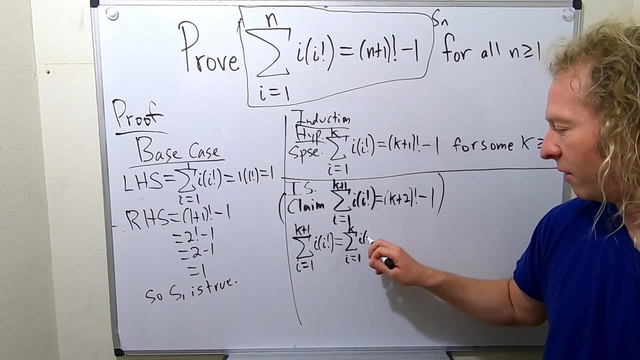 So this is the sum from 1 to k plus 1.. So a typical thing that you do with sums is you break it up, So you go from 1 to k And then you add the last piece on. So this is the sum from 1 all the way to k plus 1.. 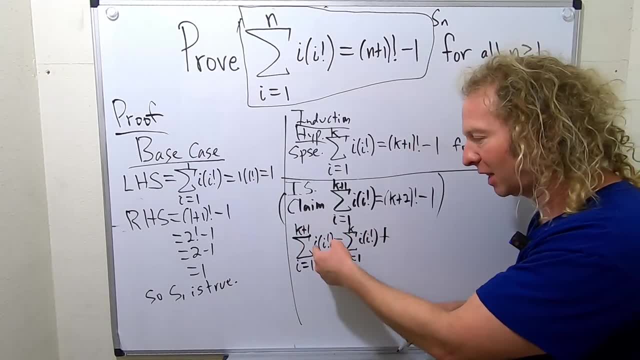 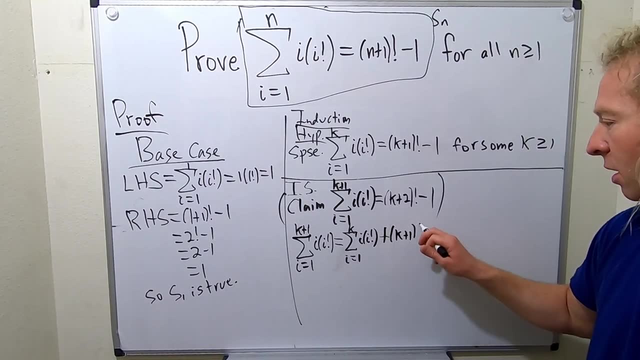 This is the sum from 1 all the way to k plus let's add that last piece, So we're plugging k plus 1 for that last piece of the sum, for that last term, It'd be k plus 1,. k plus 1- factorial. 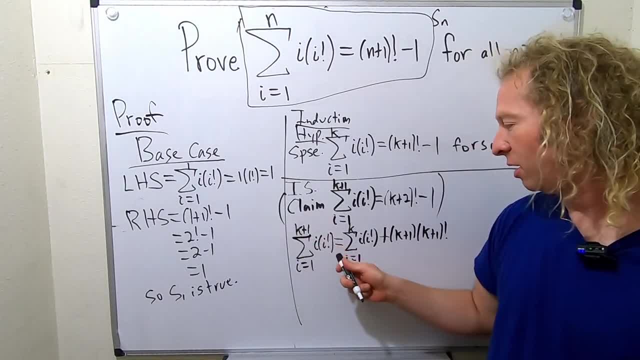 So again, this is the same as this. So here we go from 1 to k plus 1.. Here we go from 1 to k And there's the k plus 1th term. That's what that is there. Now we can use our induction hypothesis to replace this. 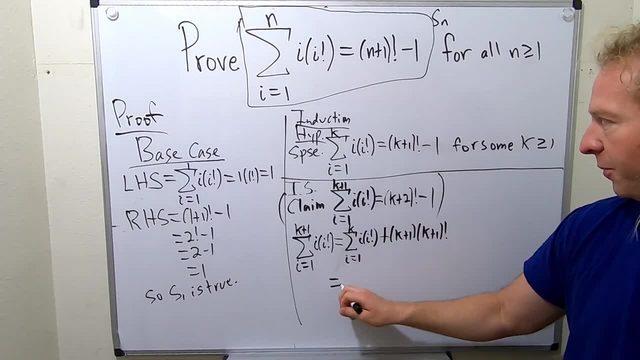 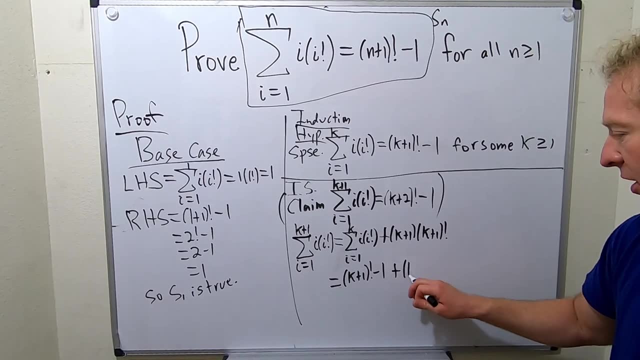 It's up here, So I'm just going to put this here. This is equal to k plus 1 factorial minus 1.. And then here we still have plus k plus 1, k plus 1 factorial. Let me pause here. 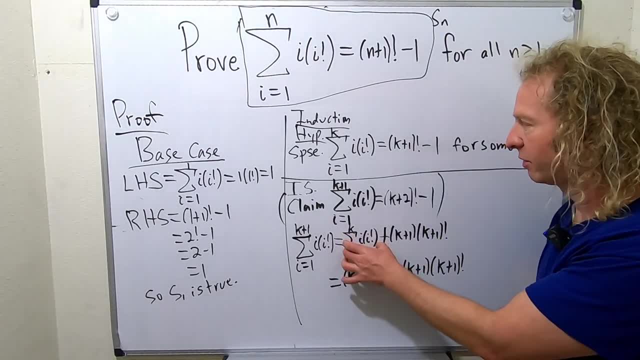 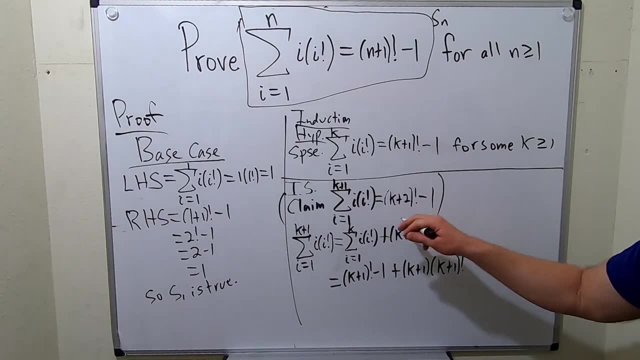 So all we did in this step is we replaced this with this. So we're here And what are we trying to do? Let's see, We're trying to show that this is true. We're trying to get this k plus 2, factorial minus 1.. 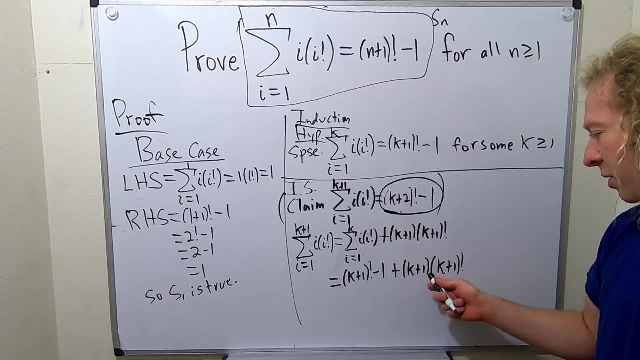 And so we're here. So you'll notice that k plus 1 times k plus 1 factorial is k plus 2 factorial. It's the same thing. However, there is another k plus 1 factorial here. So I think what we should probably do is we're going to do this. 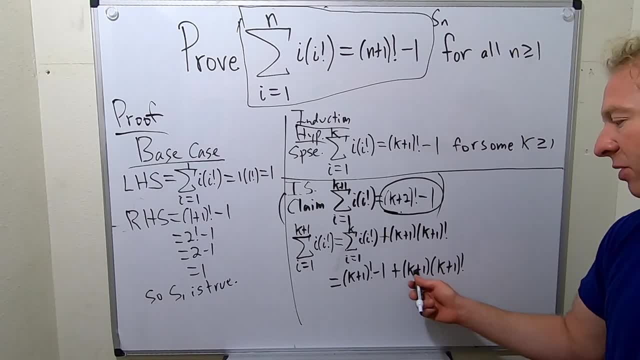 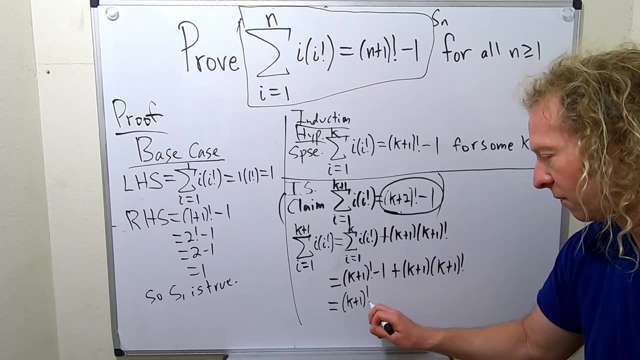 What we should probably do in this case is pull out a k plus 1 factorial, right? So let's try that. So I'm going to factor out k plus 1 factorial. I'm going to use a bracket here for added clarity. 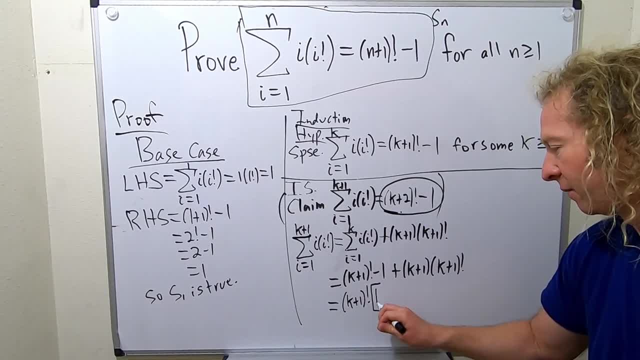 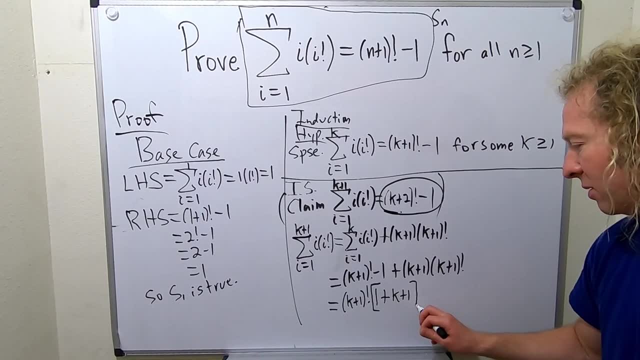 I'm trying to be really careful, So I'm going to put a 1 here. Then here we're going to be left with a k plus 1.. Going really slow. And what about this 1 here? This I'm going to put it at the end here. 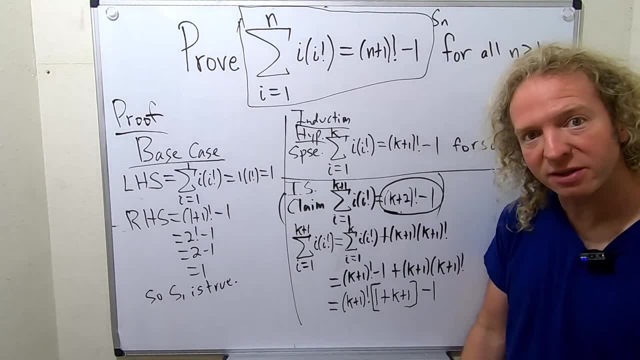 Make sure I did that right. I haven't gone through all the details of this problem on purpose, Because I feel like it's better if I show you how to do a problem as I figure it out, Because that's how you learn right. 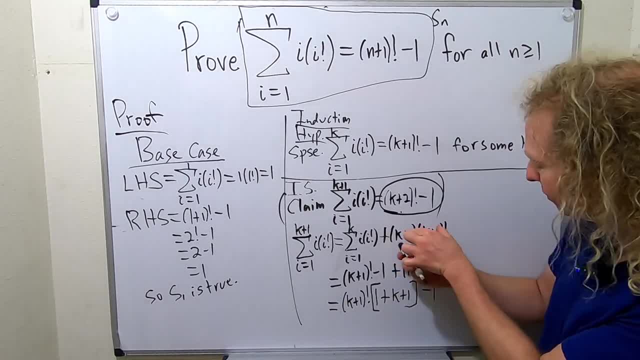 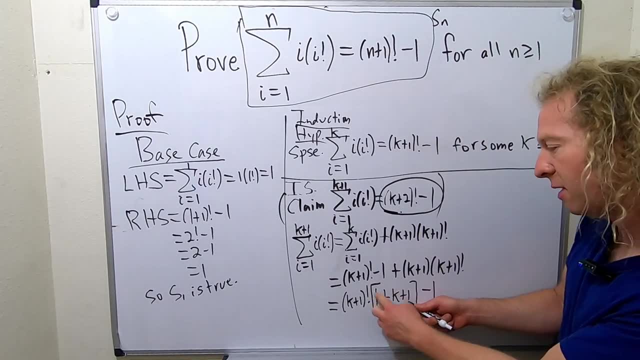 That's how you become good. So this here: pulled out the k plus 1 factorial, So you've got a 1. And then k plus 1. And then this 1 goes over here. Okay, it looks like we're good. 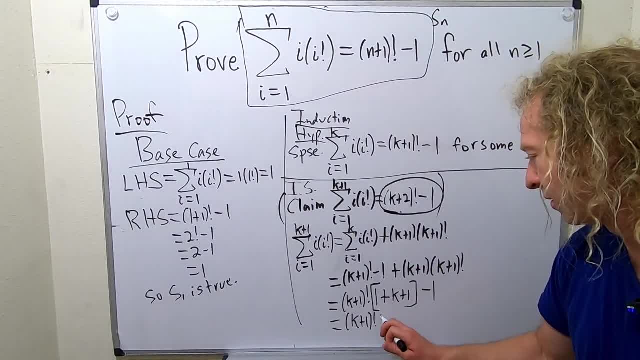 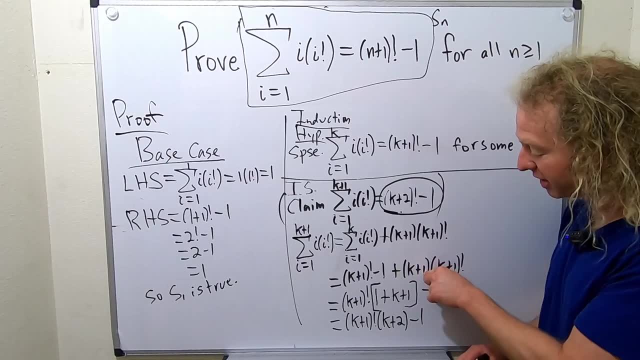 Aha, So now this is k plus 1 factorial, k plus 2.. I misspoke, by the way. I think I said something wrong. I said that this was k plus 2 factorial. It's not If that was a k plus 2.. 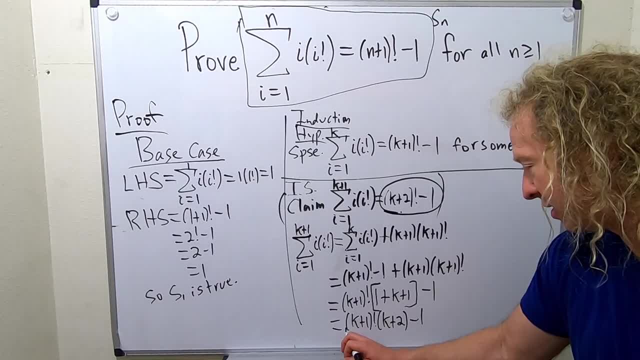 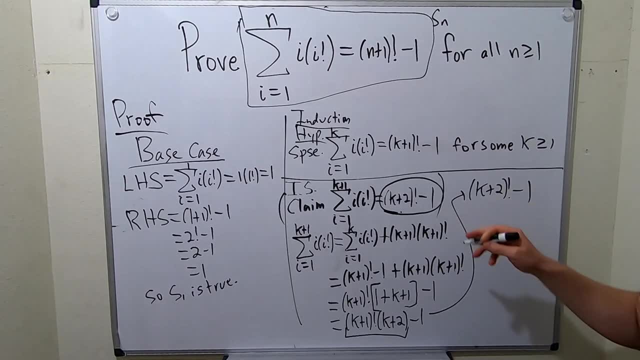 Then it becomes k plus 2 factorial right. This will be k plus 2 factorial. This is k plus 2 factorial minus 1, right. If you have n, factorial is n, n minus 1, dot, dot dot. 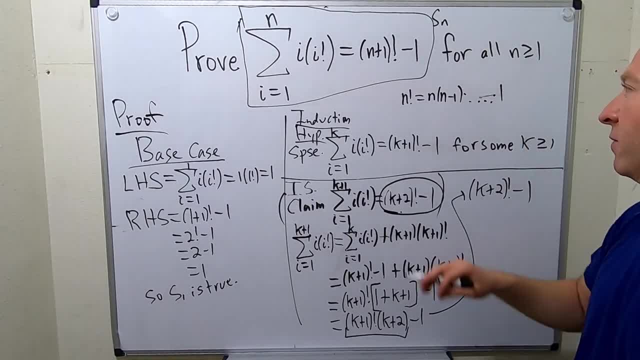 Ah, Dot dot dot times 1, right. So if you have n plus 1 factorial, that would be n plus 1, n, n minus 1, 1.. So this is actually n plus 1, n factorial. 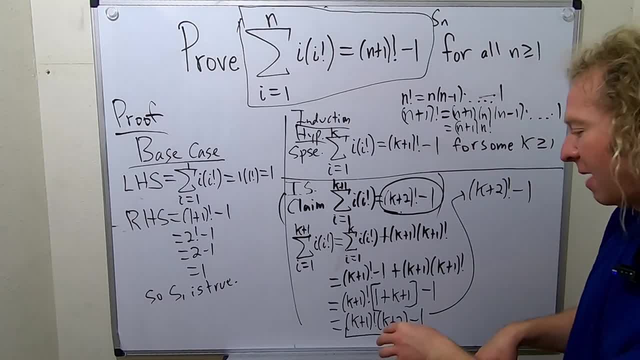 So n plus 1 factorial is n plus 1, n factorial. So the same thing happens here, right, When you have k plus 1 factorial and you multiply it by the next term, k plus 2,, you get k plus 2 factorial. 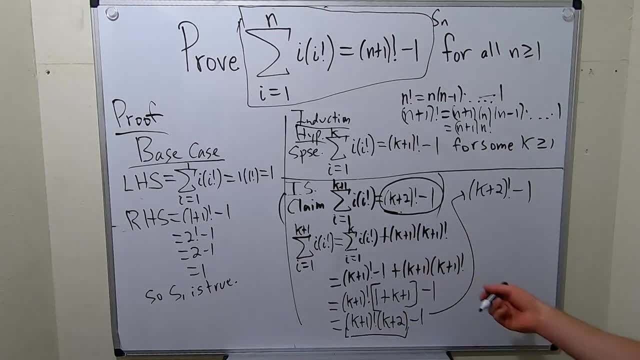 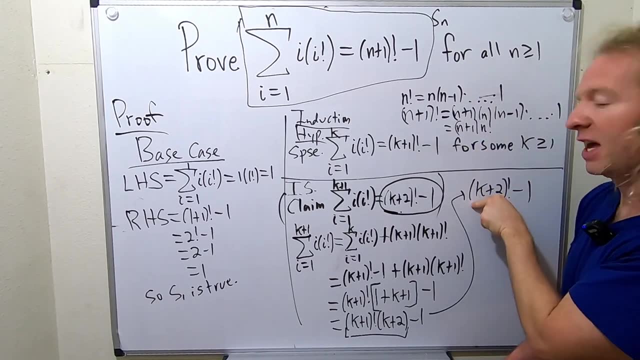 Okay, it's just something from factorials that you can do, that you need. You need this for the problem, right? So again, if you have n plus 1 factorial, that's n plus 1 times n factorial. If you have k plus 2 factorial, that's k plus 2 times k plus 1 factorial. 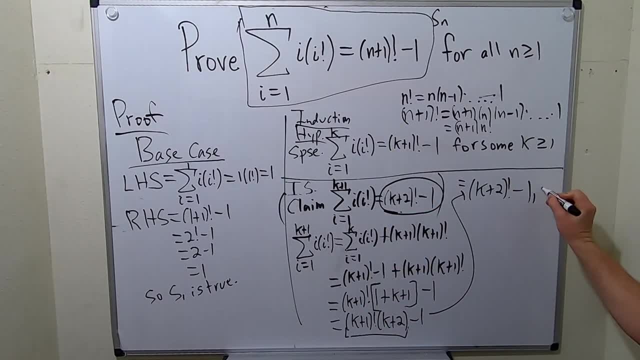 Okay, So we showed it's true, Right? So s sub k plus 1 is true. So s sub k plus 1 is true. So therefore, by PMI, by PMI, you know we are done right. 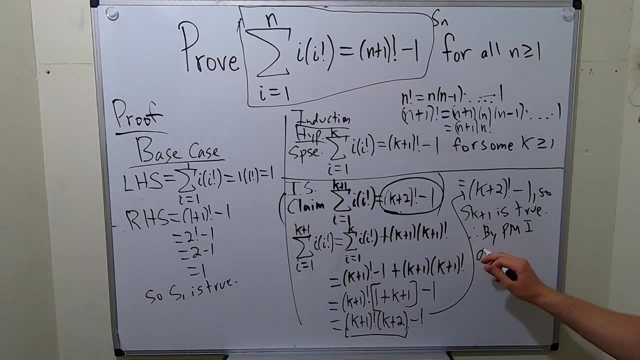 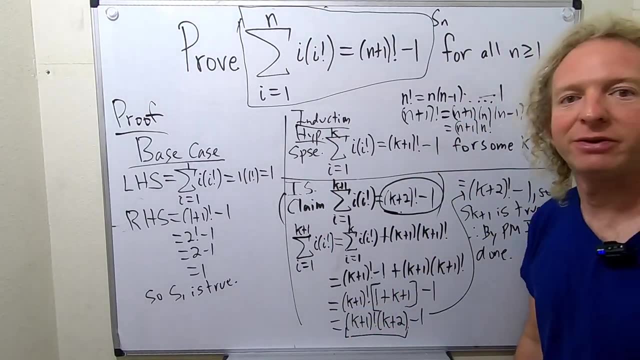 The statement is true for all positive integers: n greater than or equal to 1.. I'll say done. Yeah, You're supposed to say it right, For all n greater than or equal to 1,. we have proven it by the principle of- yeah, math induction. 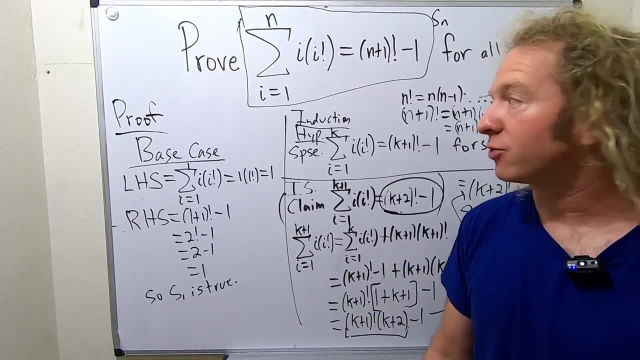 Good stuff. So interesting problem, right, Interesting problem. Yeah, that's it, Take care. 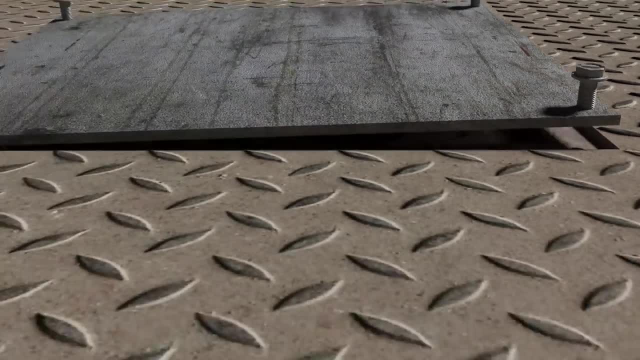 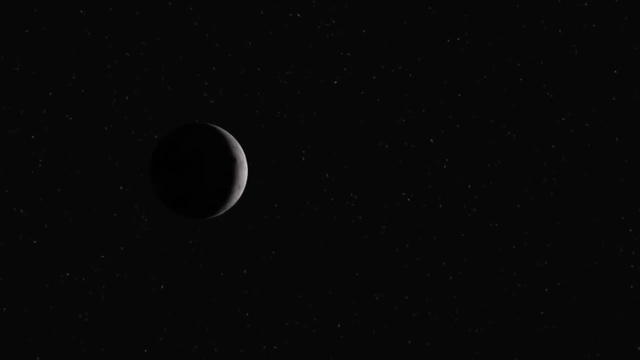 Each time you look at the moon, it's going to look a little different. Sometimes you'll see the entire moon, other times you'll see just a portion of it. In this video, I'd like to go over why the moon looks the way it does and a few other things about the moon's orbit. 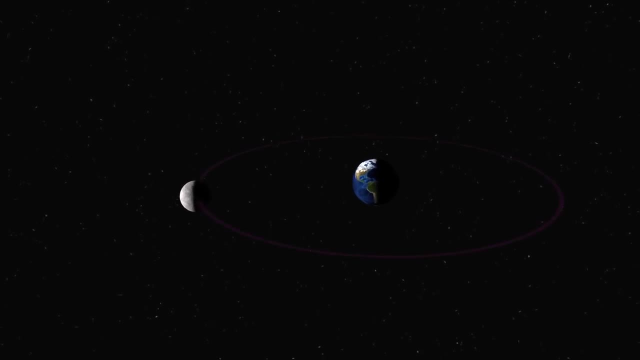 The moon takes about a month to orbit the earth. The sun can only shine on half the moon at any given time. Since the moon orbits at exactly the same rate as it spins, we only see one side of the moon from the earth. The side we don't see is usually called the far side of the moon. 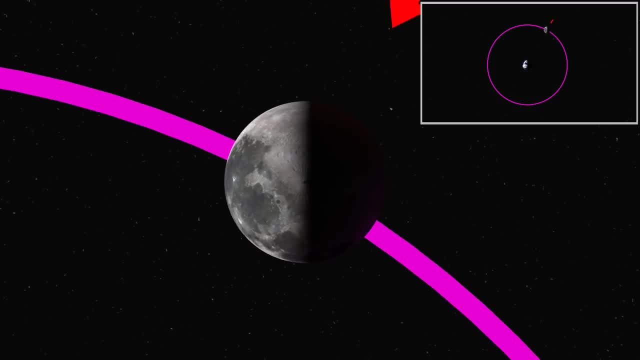 You can also call it the dark side of the moon, but it's not always dark, so this name can be a bit confusing. I'm going to show a split screen here to show you how it looks. I'll show things from two different views. 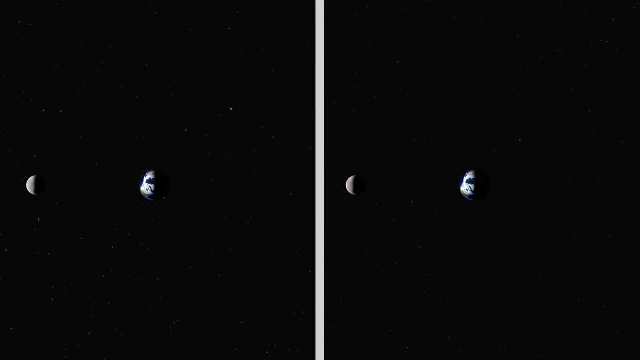 On the left-hand side of the screen, I'll show a top-down view. On the right-hand side of the screen, I'll show what it looks like from earth When the moon is closest to the sun. the side of the moon facing the earth is dark.